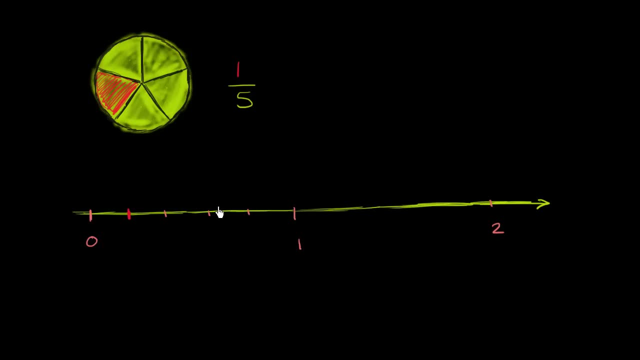 Between 0 and 1, I've traveled 1 out of the five equal sections towards 1.. And actually, let me make it a little bit neater than that, make the equal sections look a little bit better: 1,, 2,, 3,, 4, 5.. 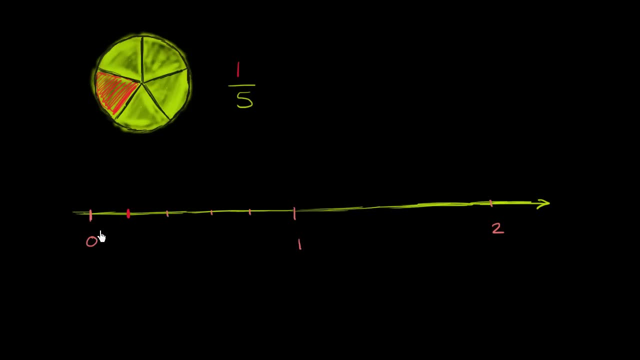 And what we're thinking about is this: What should we call this number here? This number is clearly between 0 and 1.. It's clearly closer to 0. And we've gone 1 out of the five equal sections towards 1.. 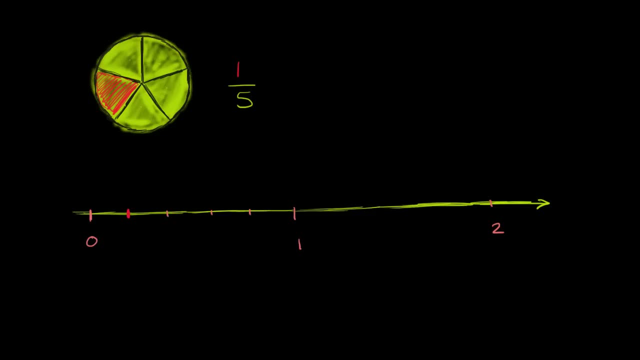 Well, it makes complete sense that. well, look, we had five equal sections here and we've traveled one of them towards 1.. So we should call this number right over here: 1 fifth. So when we're talking about a fraction, 1 fifth. 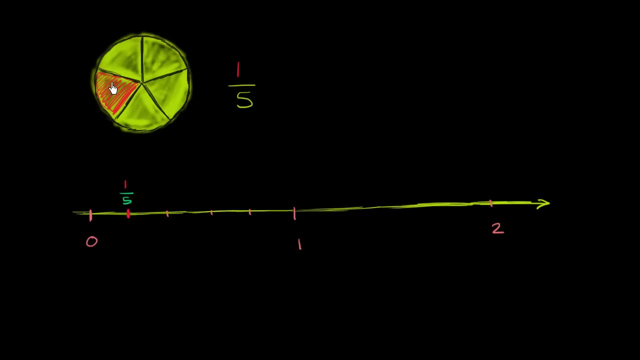 it's not just talking about, hey, what part of a pizza pie have I eaten? or something like that. This is actually a number. This is a number and we can actually plot it on the number line. Now you might say, OK, well, that's. 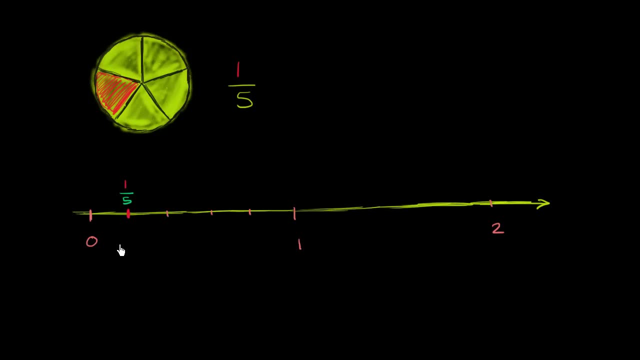 fair about 1 fifth, but what about all these other slashes? What numbers would we call that? Well, we can make the exact same idea If, up here, instead of shading in 1 out of the five equal sections, if I shaded in 2 of the five equal sections. 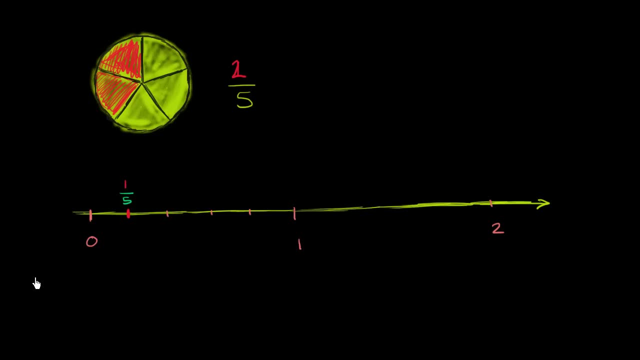 then I wouldn't say this is 1 fifth anymore. I would say that this is 2 fifths. And so if I go 2 of the equal sections towards 1, then I should call this number right over here: 2 fifths. 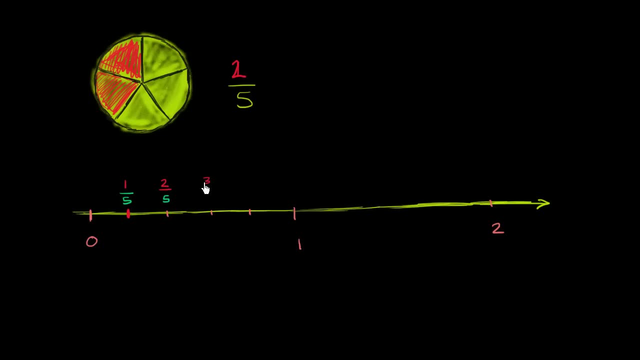 And I could keep going. This right over here should be 3 over 5.. This right over here I've gone 1, 2, 3, 4 out of the five sections towards 1.. So I could call this 4 fifths. 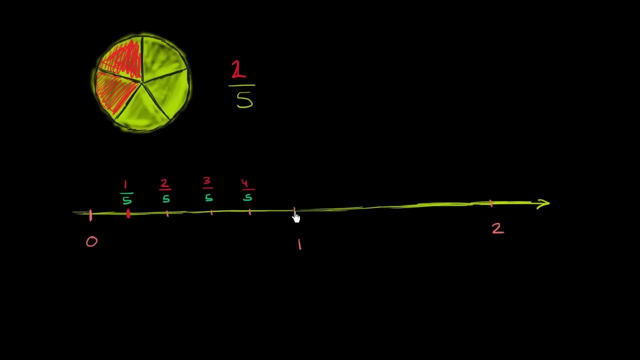 And then I could keep going. I could call this right over here. I've traveled 5 out of the 5 equal sections towards 5, so I could call this right over here: 5.. Let me do that in a red color. 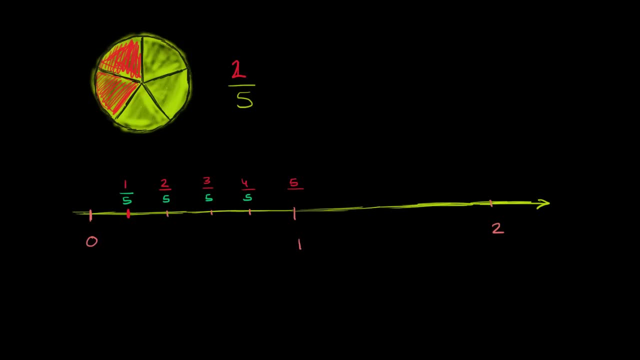 I could call this right over here, 5.. 5 over 5. And you might say, wait, but 5 over 5, we've gotten to 1. And that's exactly right. If I were to shade in 5 things over here, 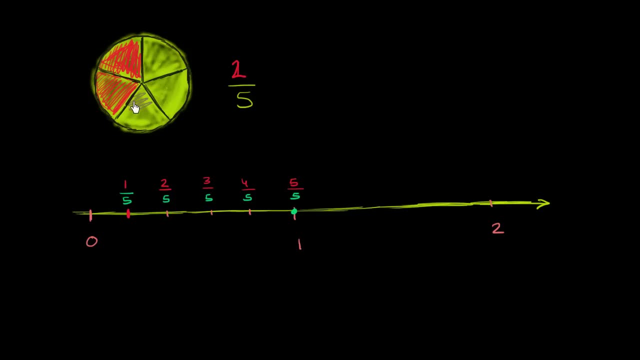 let me do that a little bit cleaner. If I were to shade in 5, that's not the color I want to use- If I were to shade in 5 things? over here we've already seen that shading in 5 things. so if this is, 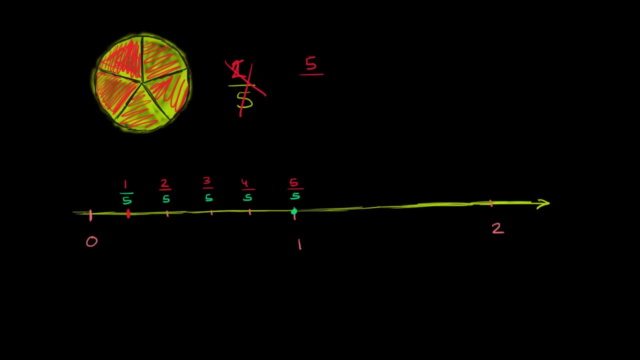 let me make this a little bit neater. if this is now 5 over 5, or 5 fifths, we've already seen that this is a whole And over here, if we've traveled 5 fifths of the way towards 1,. 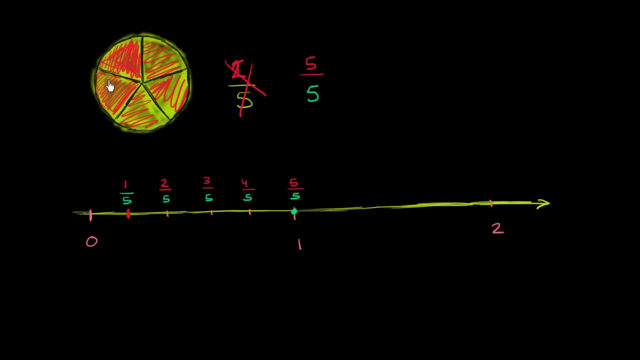 we've gotten to the whole. 1.. 5 fifths is the exact same thing as 1. It is equal to a whole. 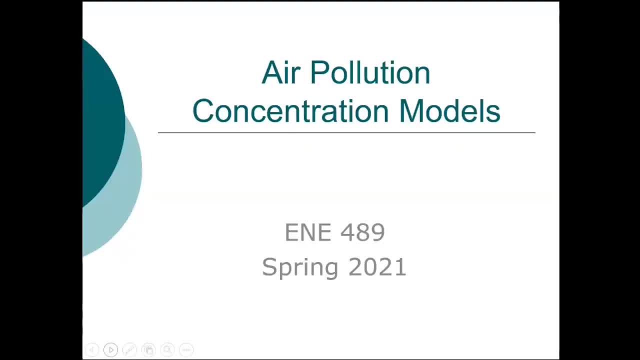 Okay. so what I would like to do today is move on to the air pollution concentration modeling unit, And what we will do in this unit is we'll initially start with looking at box models And then, from the box models, we will look at Gaussian dispersion. So in